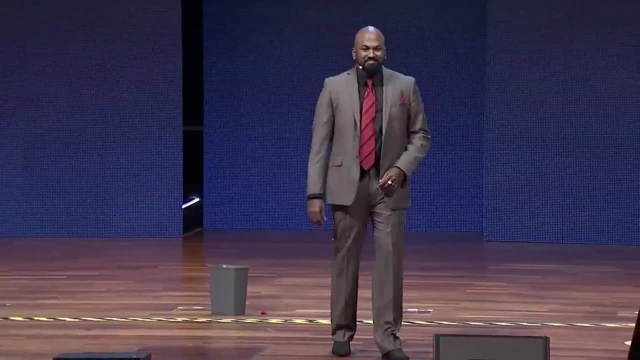 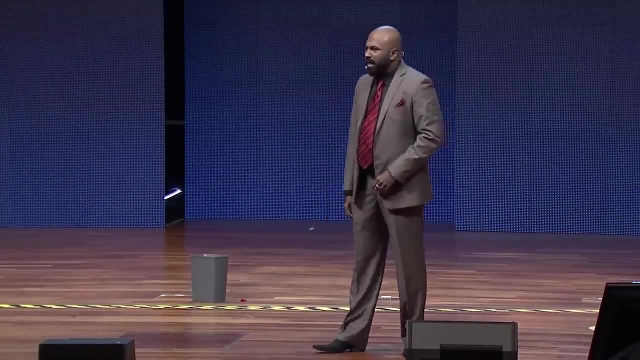 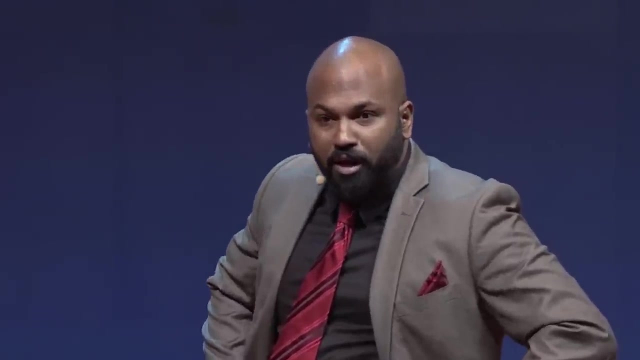 Mr Cottage Chair, My fellow flowers. I can remember the first time I broke, I was 17 years old. I had already flunked high school and managed to get myself arrested. Now, I wasn't afraid of the cops, But there was one person I was very afraid of. 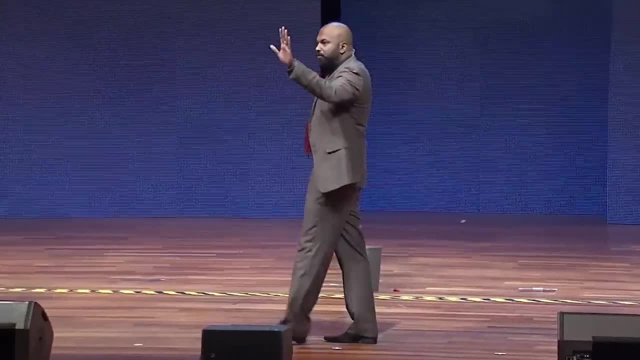 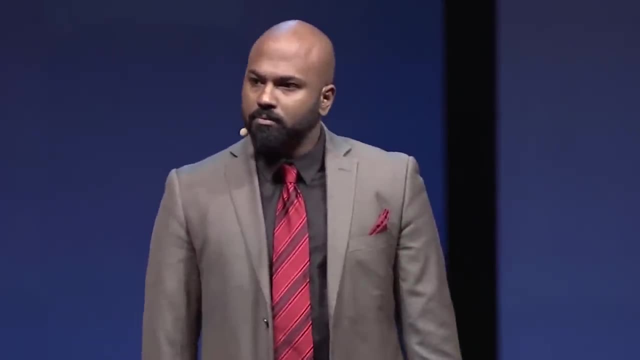 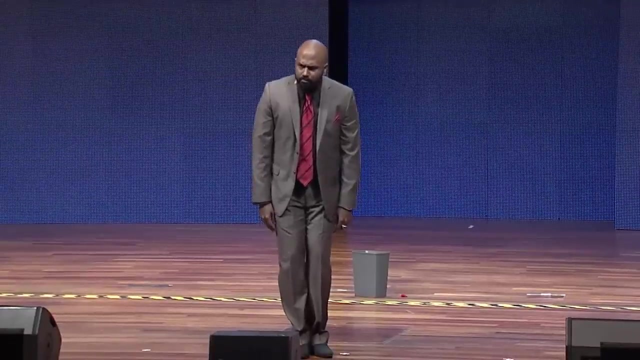 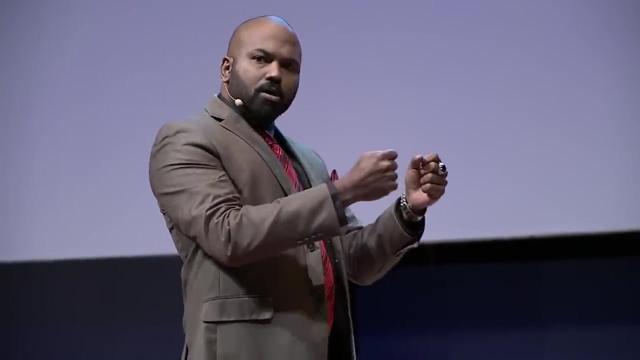 And that was my mama. Raise your hand. if you have an emotional mother, Let me see. Put them all together, you get mama. I can hear her scream outside the police station. Even the cops were afraid. She came up to me, held the iron bars, looked into my eyes and I saw a tear coming down her face. 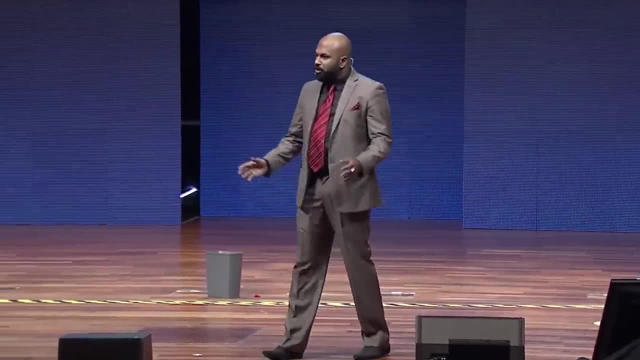 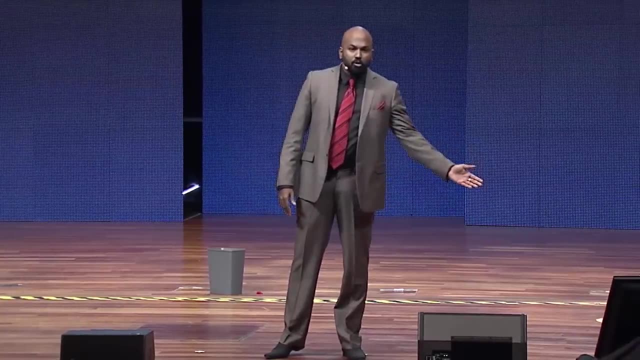 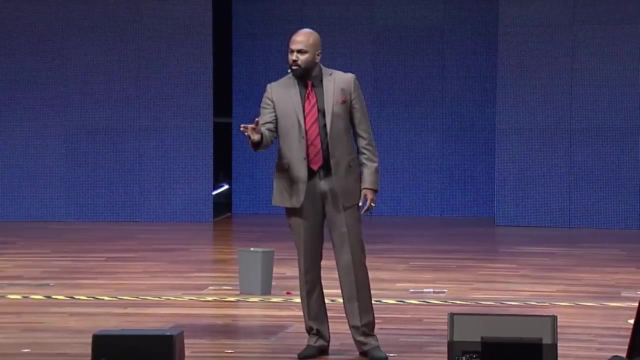 Now, I've seen my mama cry before, But mothers cry three types of tears: Tears of joy, Tears of sorrow And tears of shame. And when a son sees a mother cry tears of shame, that's a life-changing moment. She looked at me and said: son, I want you to be a better man. 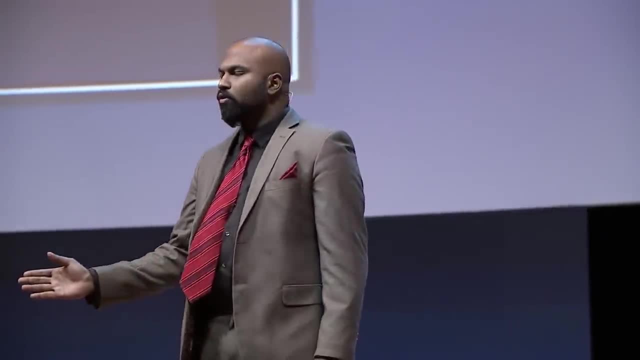 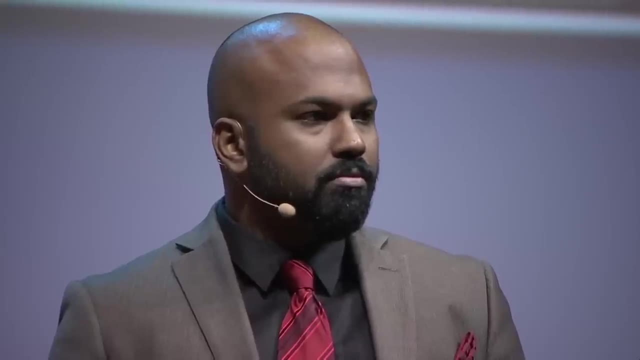 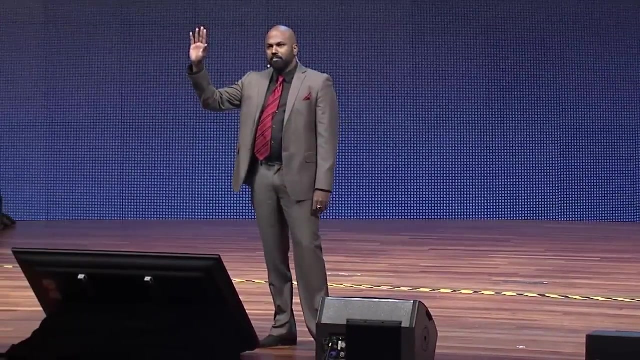 That night, when I drove home, my dad was waiting for me at home. Now, my dad is a cool dad. Raise your hand. if you have a cool dad, Put them all together, you get my dad. My dad came up to me and said: son, it's okay. 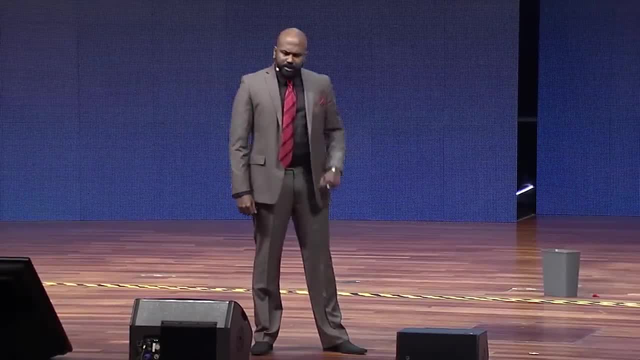 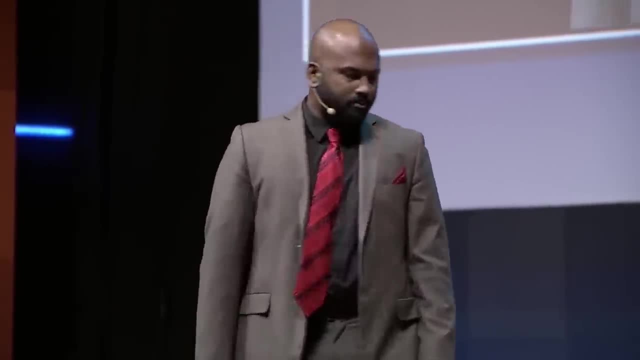 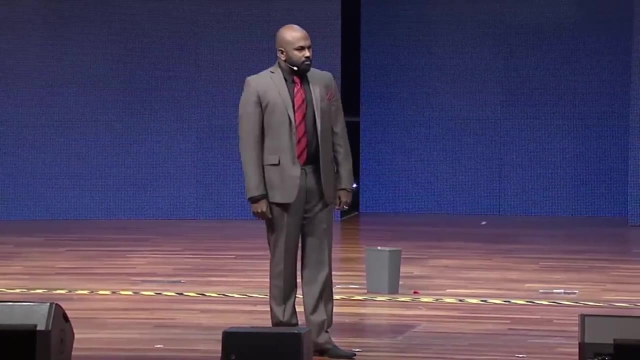 You flunked your exams. You already got arrested. That's fine, You get that from your mother's side. I want you to start working immediately, And I said okay. So my dad took me to meet one of his friends called Sam. 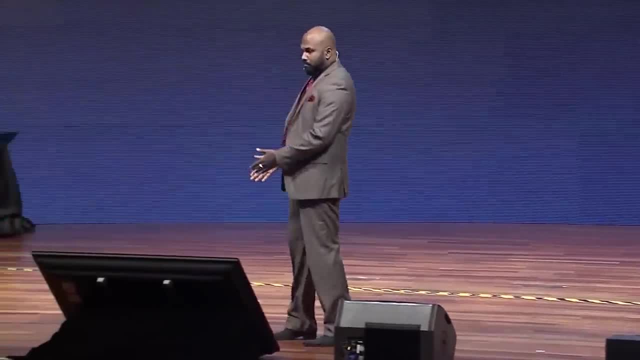 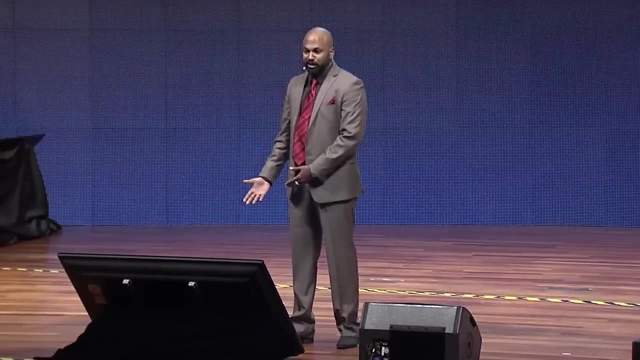 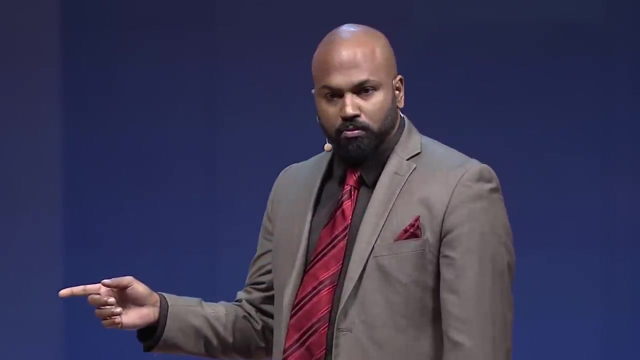 He said: I want you to be a better man Now. Sam was an accountant who had an accounting firm and had generously decided to make me his personal assistant. And there he was. He looked like a teddy bear, But this man was special. 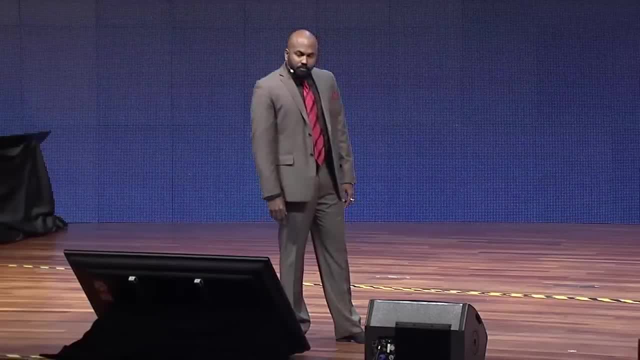 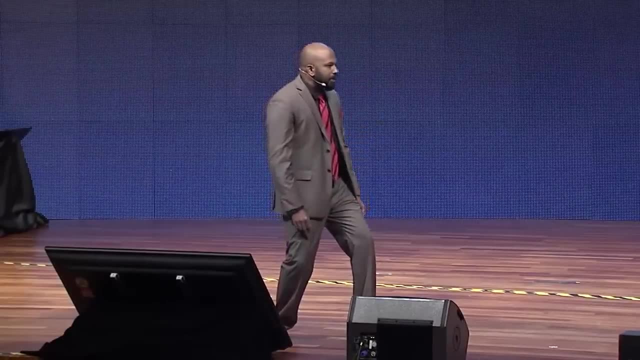 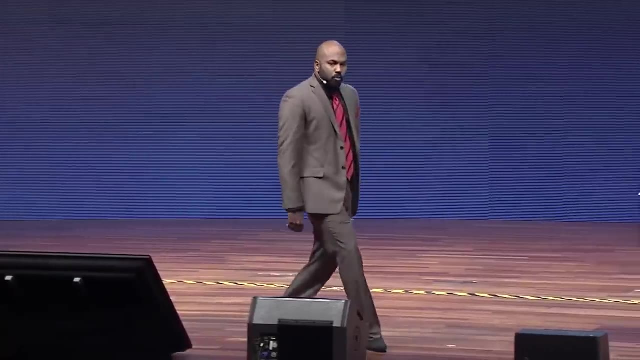 I looked at him and he looked at me, And then he said the most amazing thing. He said, son, I see something in you, But I don't know what it is. If you decide to work with me, I can help you find that something. 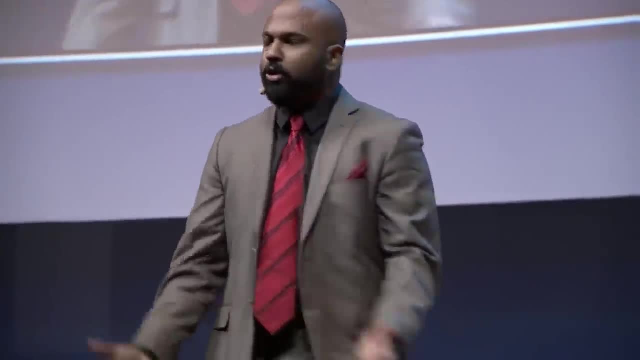 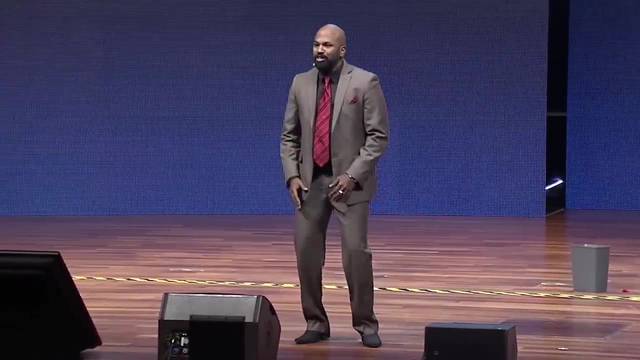 And I was like whoa, that's the first time in my whole life somebody has ever told they see something in me. And I started working for Sam And every day after work, he used to tell me stories about the world, about history, about culture, about philosophy. 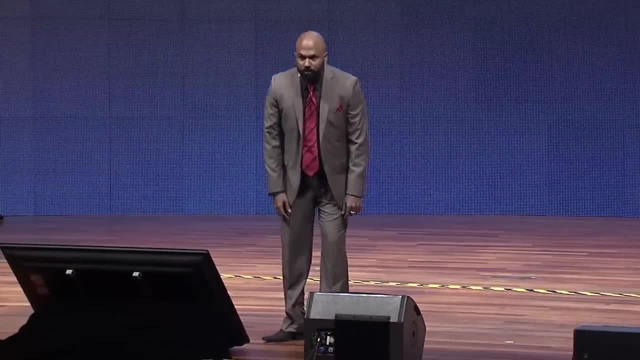 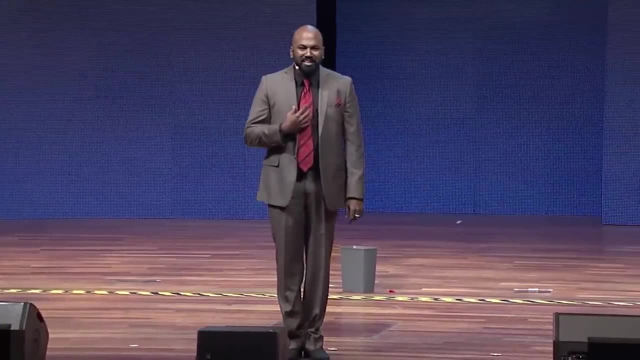 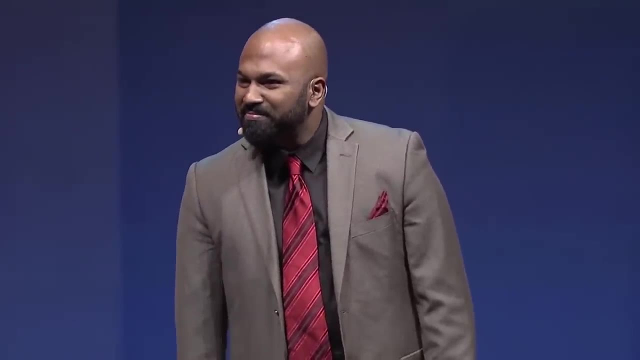 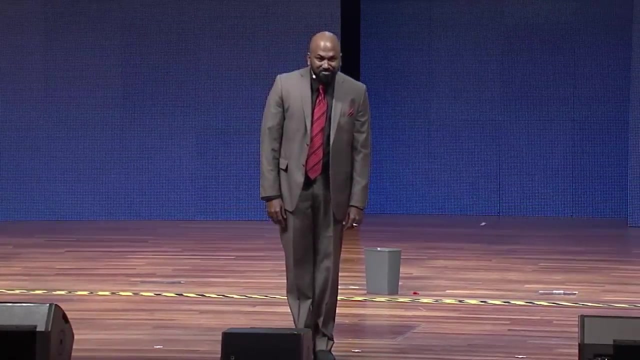 And it was much more interesting than what I learned in school. And I discovered I can dream. And I started dreaming. ladies and gentlemen, After one year, I went back into high school, completed my exams and went into college. After successfully completing college, I found a great girl. 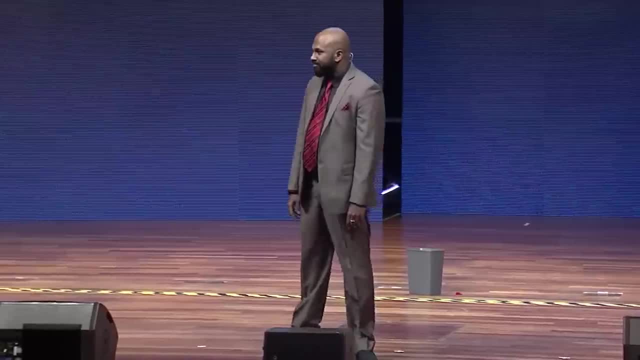 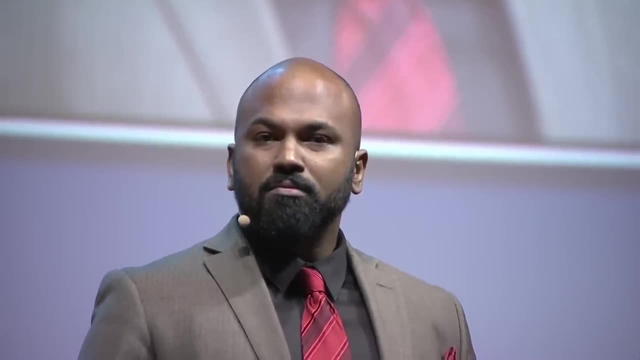 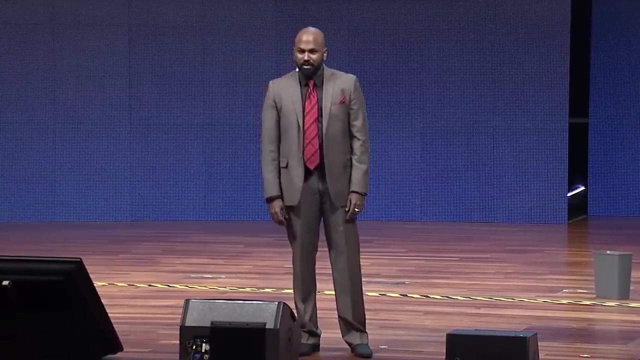 But not a job. I didn't know what I wanted to do with my life. Have you ever had that problem? And when you're lost it's difficult to feel special. So I went back to my cool dad And I said, dad, I feel lost. 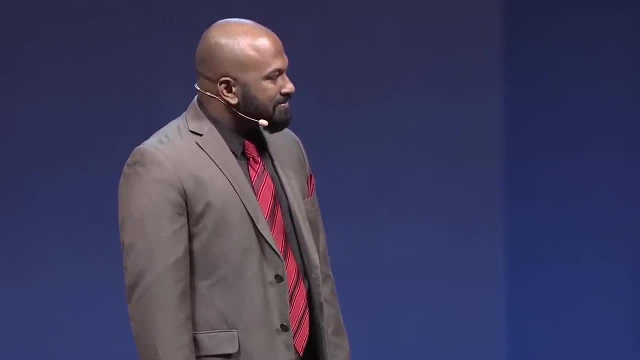 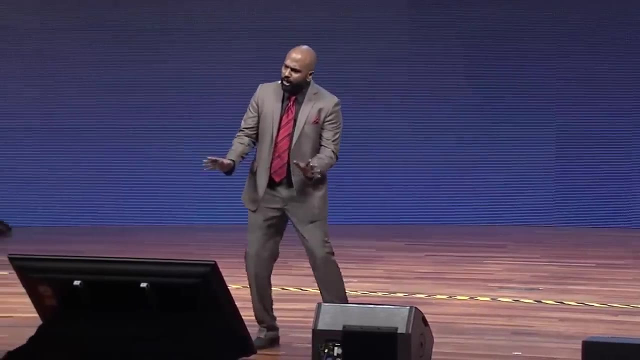 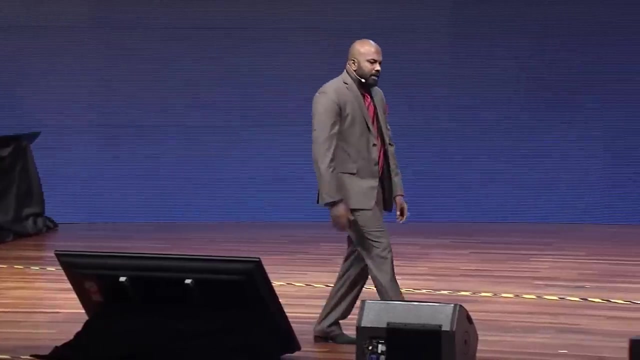 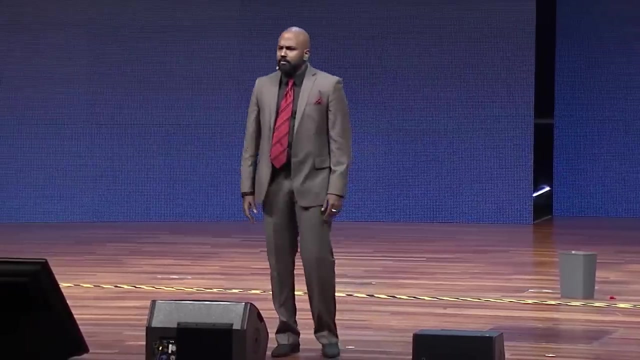 He said: you are like your mother. So my dad introduced me to this strange club that had a strange name, with strange people talking. On the first meeting they told me to do something called a table toppling. I aced it, But while I was speaking I see a strange man seated in the back row. 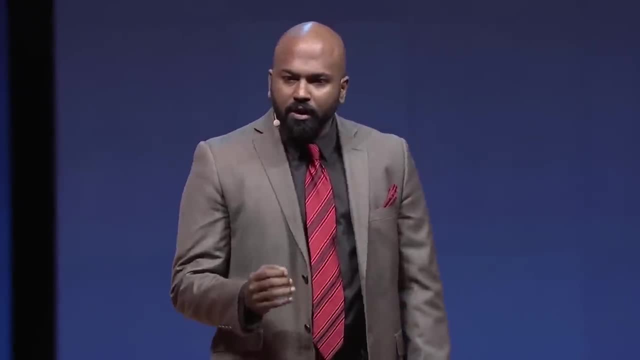 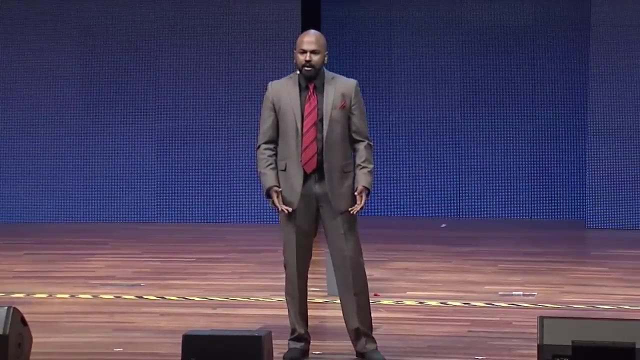 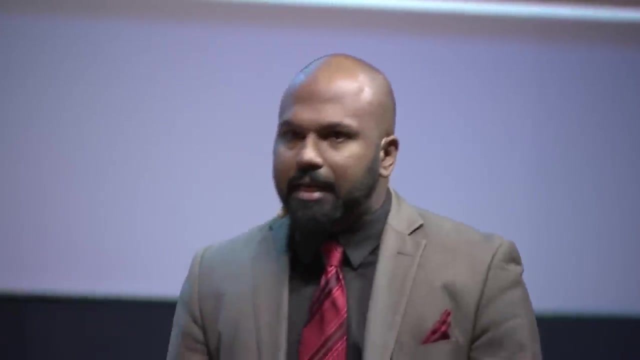 Humble, simple, The unfailing quality of kindness in his eyes. As soon as I finished, he walked up to me, looked me dead straight in the eye and said: son, I see something in you, But I don't know what it is.